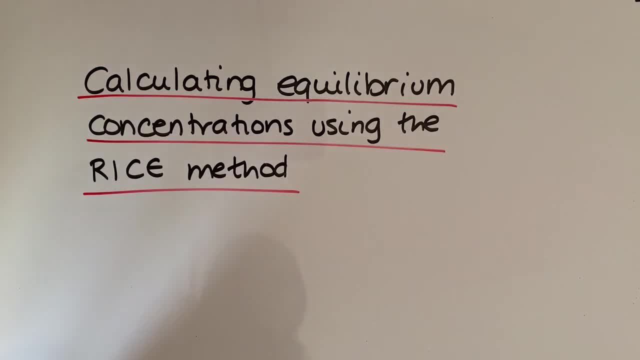 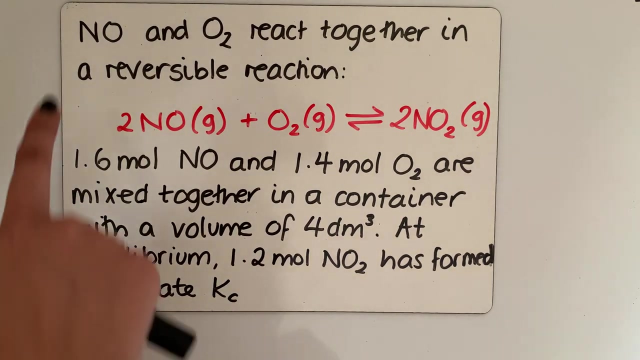 So what we now need to do is use something called the Rice method to calculate the equilibrium concentrations and then plug that into our Kc expression to get Kc. Now, in order to do this, I need to do this with a question. So I have a question over here. We've got nitrogen monoxide and oxygen reacting together in a reversible reaction, with the balanced equation here. 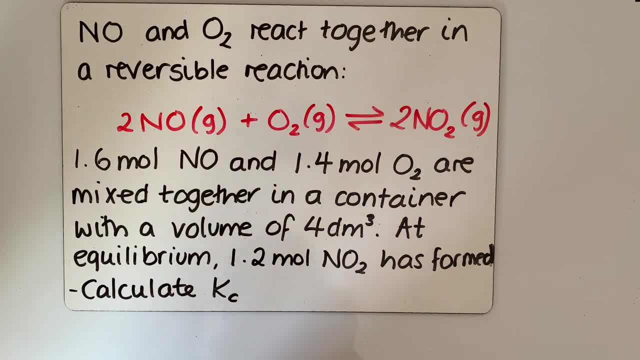 We're then told that 1.6 moles of nitrogen monoxide And 1.4 moles of oxygen are mixed together in a container with a volume of four decimetres cubed. So now we're not given the equilibrium concentrations and we are given the initial moles of everything. 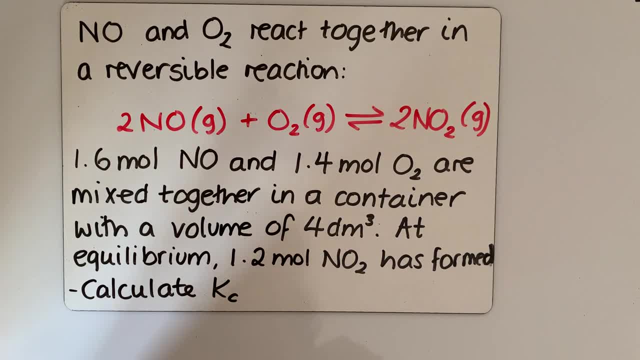 OK, and we've got the volume of the container which is going to come in handy at the end. And at equilibrium we have 1.2 moles of nitrogen dioxide being formed. So we're given the equilibrium moles of the product. 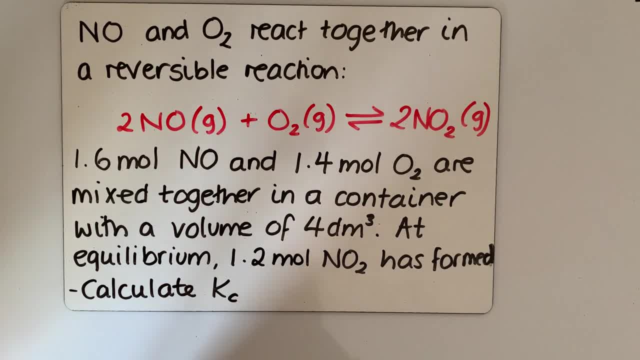 OK, so essentially What we need to do now is work out the equilibrium moles of everything, of the reactants, and then from there work out the equilibrium concentrations, And once we've done that, we can then plug that into the Kc expression to get Kc. 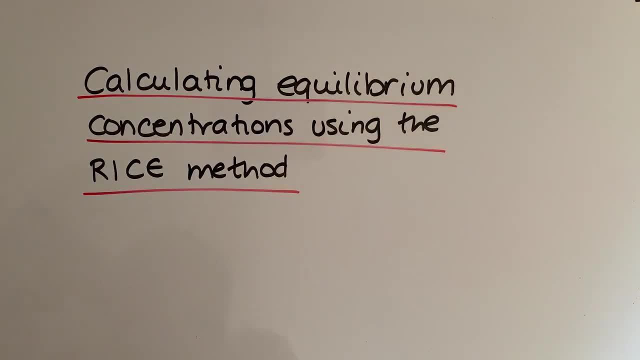 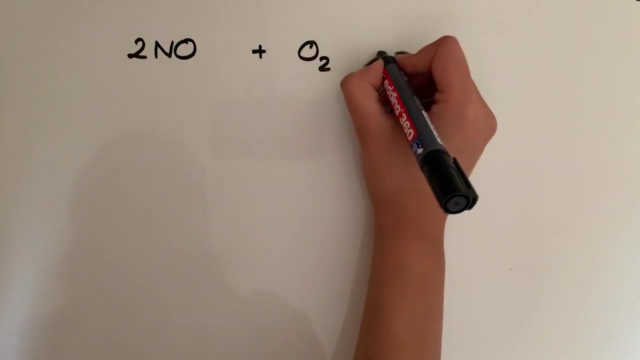 OK, so I'm going to show you how you should set out your working out for the Rice method. The first thing that I do is I write out the balanced equation slightly more spread out. So it's 2NO Plus O2 goes to 2NO2.. 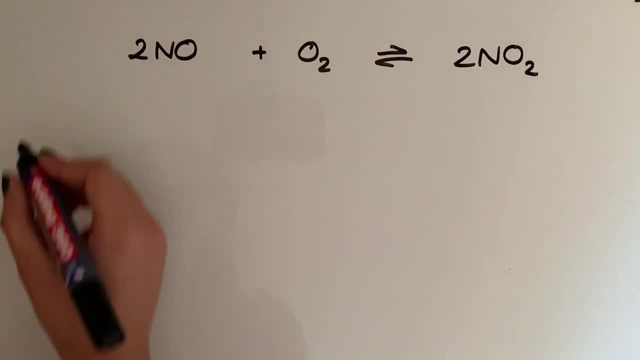 OK, and then, along the left hand side, I'm going to write our Rice and I will explain what each of them stand for. OK, so Rice, And, as you see, we're going to kind of do some working out over here. 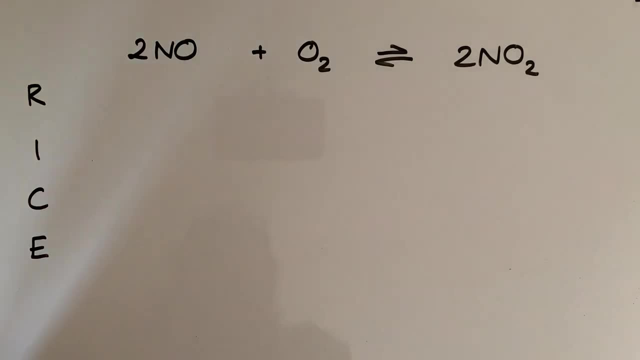 So this is how you should set it out. So the R in Rice stands for the ratio of moles, OK, so I'll just write that here. So it's a ratio of moles, OK, and we just get that from the balanced equation. 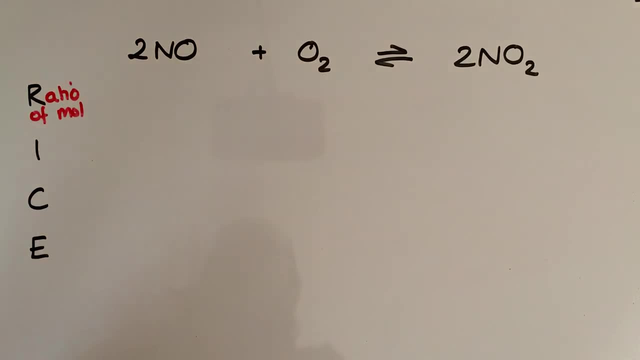 OK, so all we do is we look at the balancing numbers and that gives us our ratio of moles. So over here balancing number for nitrogen monoxide is 2.. For here it's just 1., And for nitrogen dioxide it is 2.. 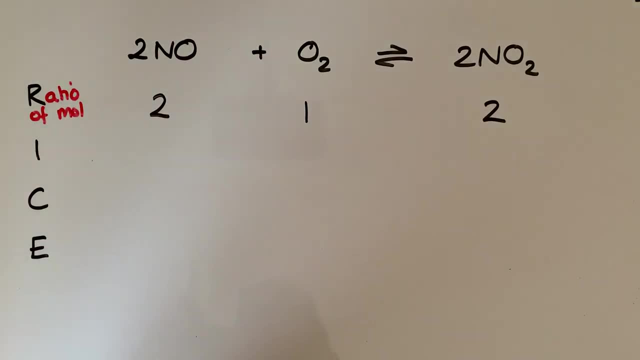 OK. so this is the ratio of moles based on the balanced equation. OK, next thing: The I It stands for initial moles, OK, and the E stands for equilibrium moles, OK. so the moles at the beginning and at the end we have our equilibrium moles. 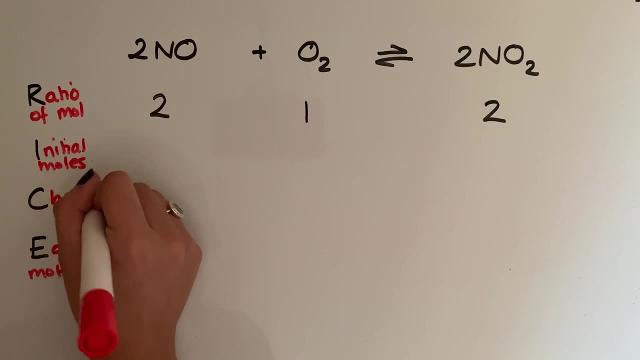 And the C stands for the change in moles. OK, so let's now have a look at how this applies to this question. So, if I just grab the question again, what we want to do just by using. So, if I just grab the question again, what we want to do just by using: 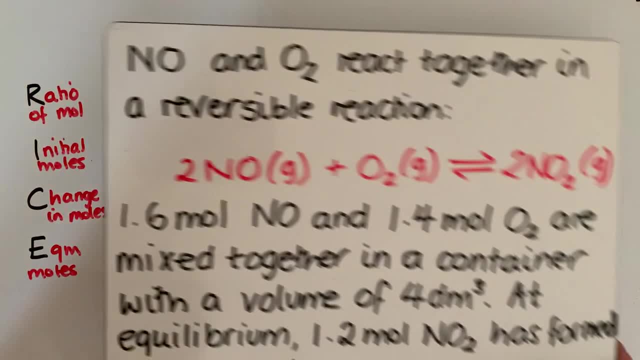 So, if I just grab the question again, what we want to do just by using Fill in parts of this rice table? OK, so we're told we have 1.6 moles of NO and 1.4 moles of O2 at the beginning. 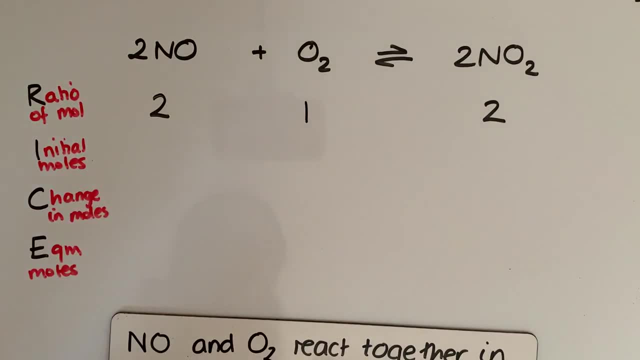 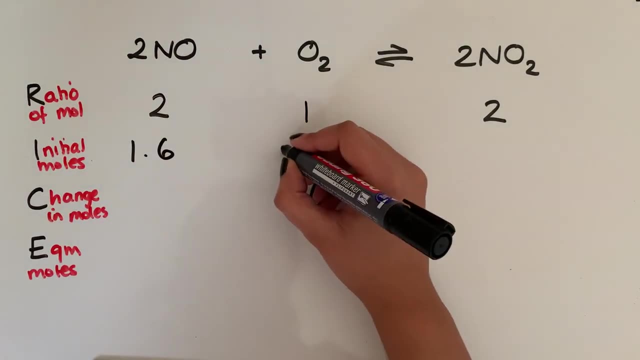 OK, so the initial moles for nitrogen monoxide is 1.6 and the initial moles of oxygen are 1.4.. OK, so, before the reaction even starts, this is how much nitrogen monoxide and this is how much oxygen. 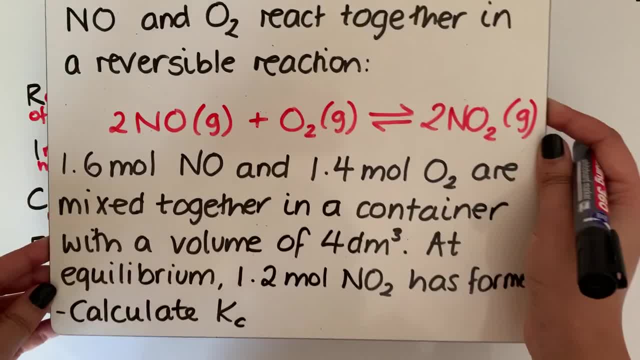 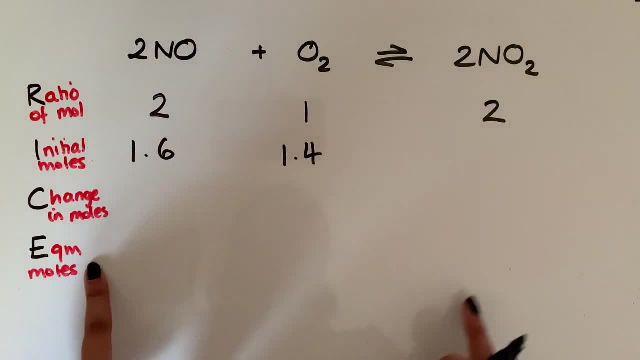 We have OK, and then we're told: at equilibrium, 1.2 moles of NO2 have formed. OK. so at equilibrium we have 1.2 moles of NO2.. So I'm going to put 1.2 moles of NO2 there. 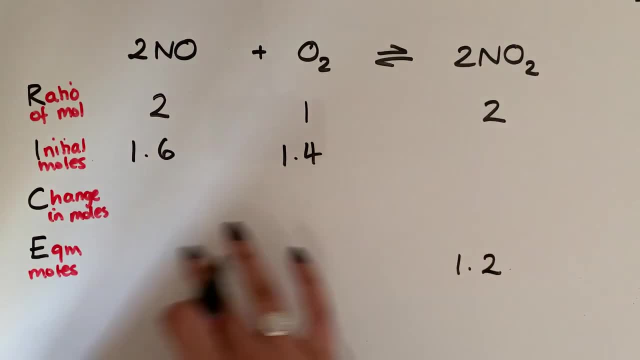 OK, and this is what we get just from the question, And we now got to basically work out all the gaps. So it's worth noting that at the beginning you are only going to have So, before the reaction has even started, you are only going to have reactants. 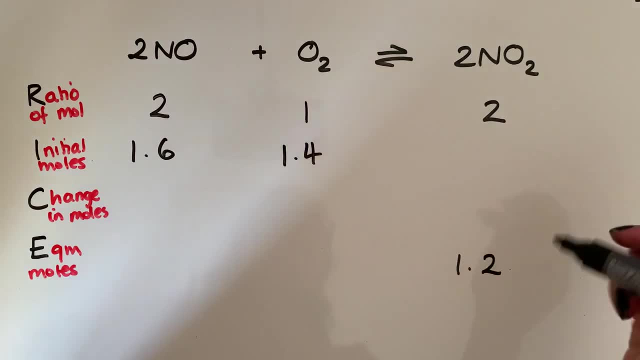 You are going to have no product. So the moles of the product, the moles of our NO2, are going to be zero. OK, we never have products at the beginning. Now, or in this reaction, we don't have any products at the beginning. 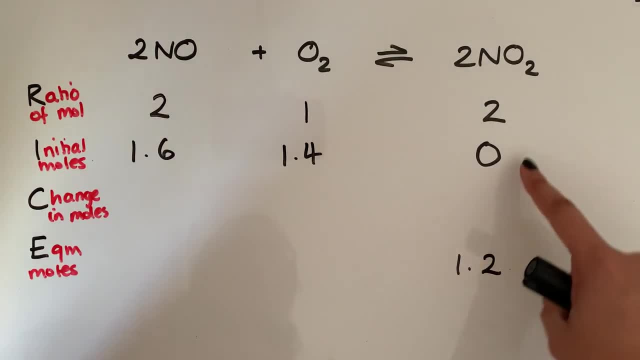 OK, what we're now going to do is we can now look at the change in moles. So over here, this is the only one where we know the initial moles and the equilibrium moles, So we can essentially work out the difference between the two. to look at the change in moles. 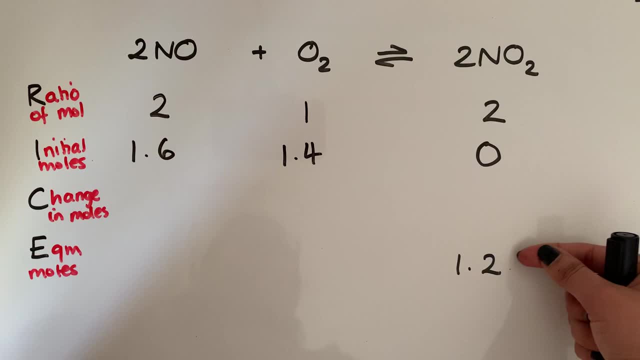 OK, hopefully you can all see that the change in moles is Plus 1.2.. So, to go from zero to 1.2, we have added 1.2 moles. OK, it's also worth noting that in this one and most of them, we are going to gain products and we're going to lose reactants. 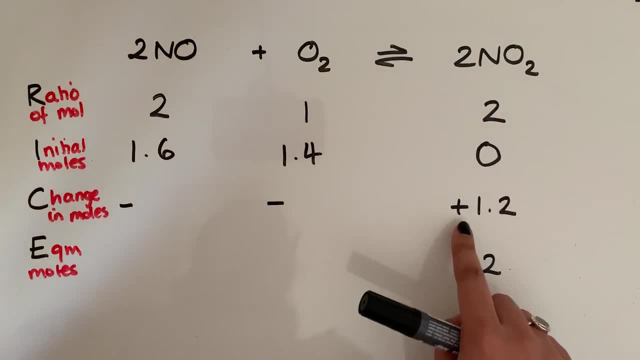 So we're always going to lose reactants and we're going to gain products. OK, now we need to look at what the change in moles are going to be for our reactants, And this is where the ratio of the moles is. 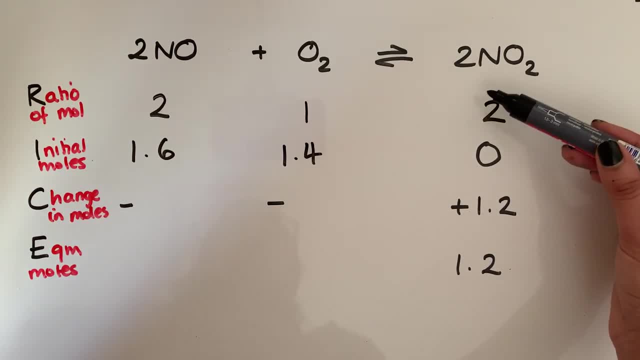 This is where the ratio of the moles is going to be important. OK, we're saying that nitrogen dioxide is worth two moles, So that gained 1.2.. OK, so if we want to look at one mole, so one mole is going to be half of that. 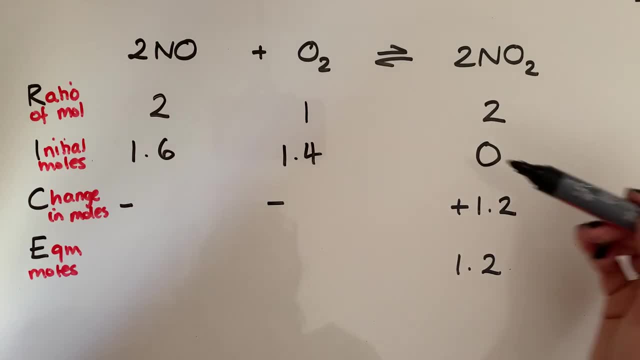 So one mole is just going to be 0.6.. OK, so over here we have one mole. We just said one mole is 0.6 based on the ratio of these two. So for O2, because it's our reactant, we're going to lose it. 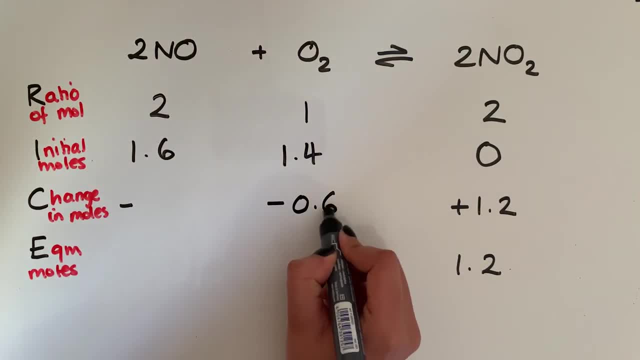 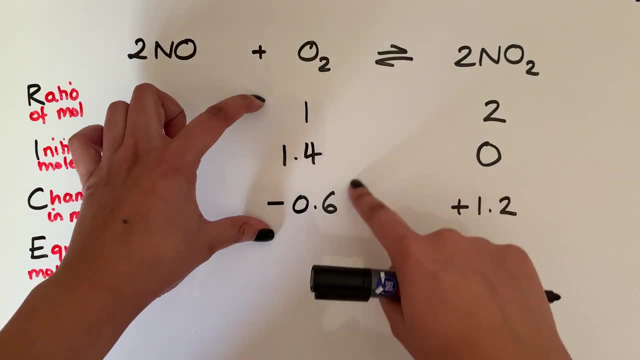 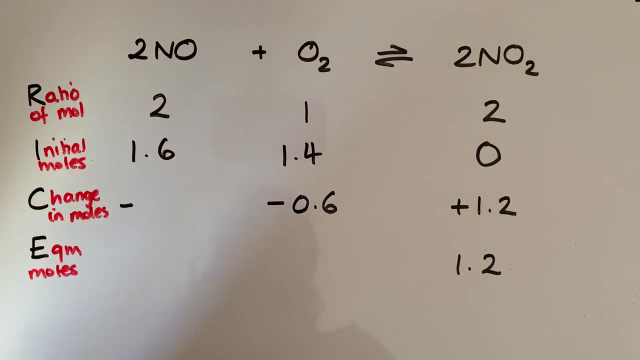 We are going to lose it. We are going to lose 0.6 moles, OK. so these ratios need to make sense over here. So two is 1.2.. One is 0.6.. It's negative here because we're losing reactants, and positive here because we're gaining products. 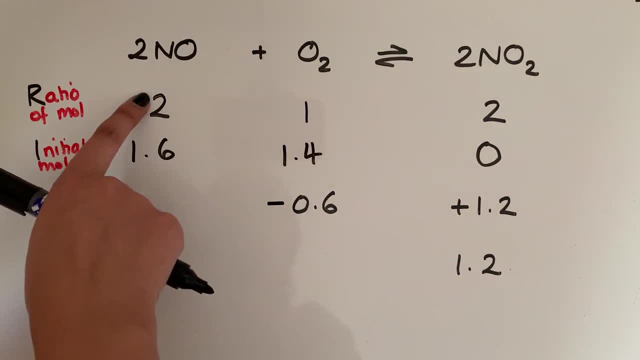 OK, if we now go to NO, this is now two, So two is worth 1.2.. So we're now going to lose 1.2 moles here, OK, So now all we're going to do is we're going to apply those changes to get the equilibrium moles down here. 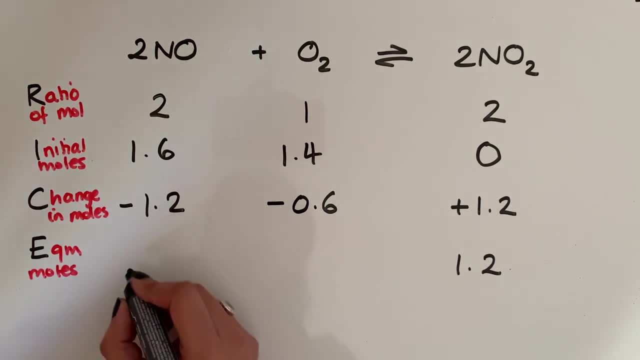 So we're going to do 1.6 minus 1.2, which means we're left with 0.4.. And then over here we're going to do 1.4. take away 0.6.. So that means we're left with 0.8.. 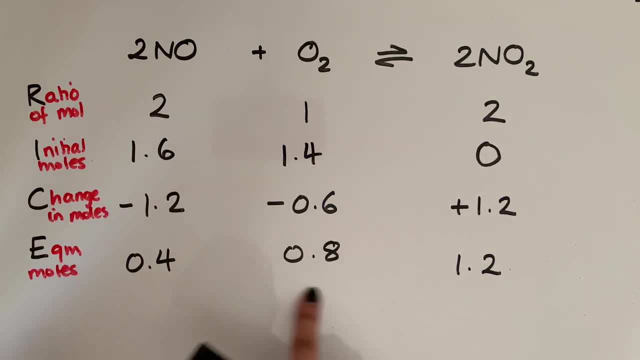 OK, we now have our equilibrium moles for everything. OK, so we're nearly there. We can nearly start plugging things into KC. except in KC we plug in concentration, We don't plug in moles. So to go from moles to concentration, remember the units for concentration are moles per decimetre cubed. 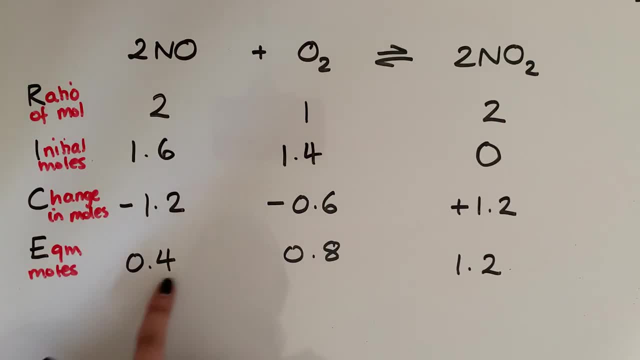 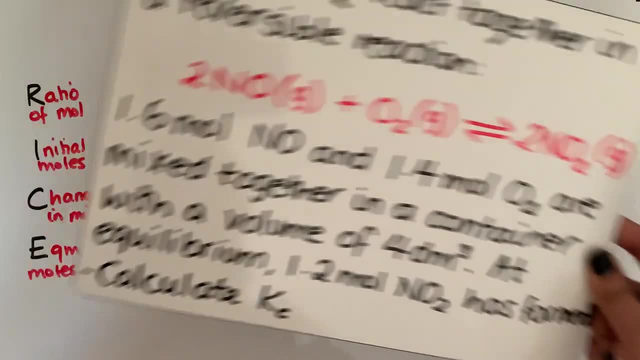 So to go from moles to moles per decimetre cubed, we're going to divide everything by the total volume. Now, if you remember, in the question it said the container had a volume of four decimetres cubed. 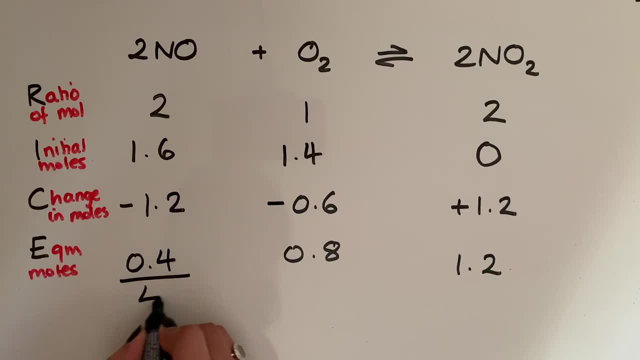 So all we're going to do is divide everything by four decimetres cubed, And that's going to give us our concentration in moles per decimetre cubed. So this one here is going to equal 0.1 moles per decimetre cubed. 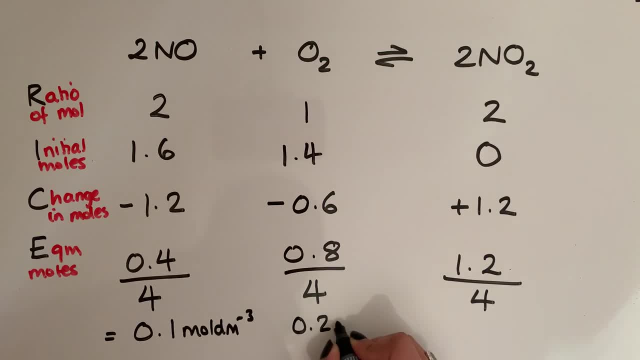 This one over here is going to equal 0.2 moles per decimetre cubed, And this one's going to equal 0.3 moles per decimetre cubed. OK, so we now have our equilibrium concentrations. 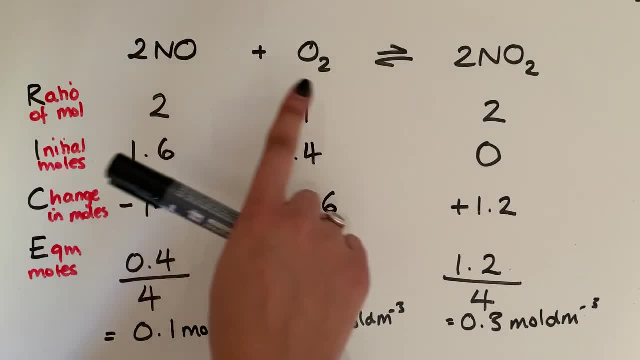 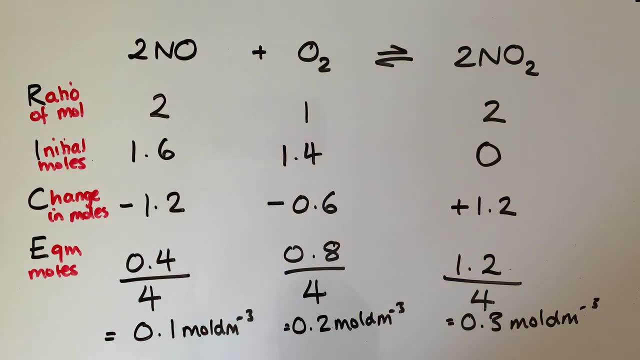 So these are our equilibrium concentrations And for each of these species. OK, what we're now going to do is we're going to plug those values into our KC expression, But firstly we need to write our KC expression. I'm just going to leave these values down here. 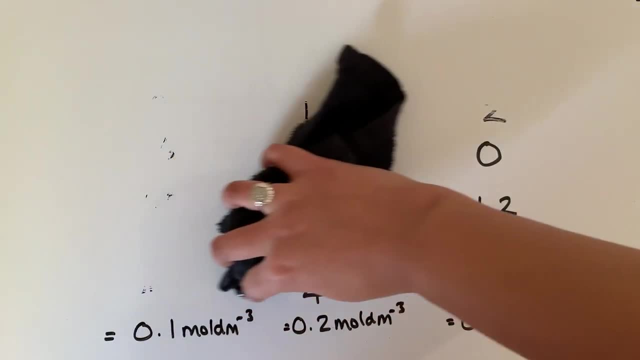 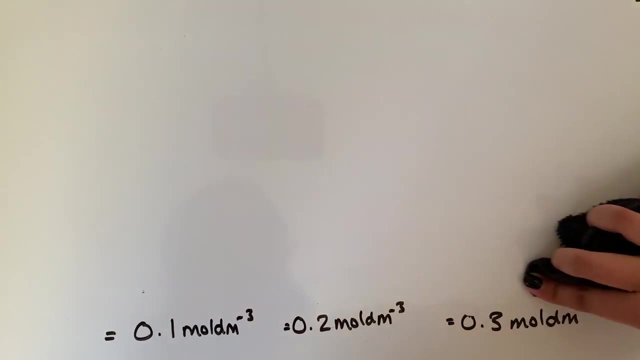 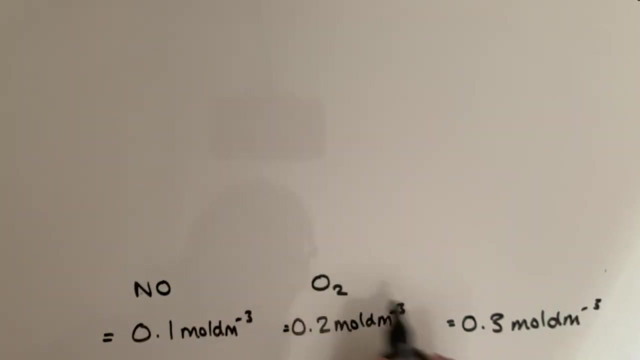 I'm just going to go back the top. OK, so just to remind you, this one is for NO, This one is for O2.. And this one is for NO2.. OK, right, So KC expression. if I just write out the balanced equation again, 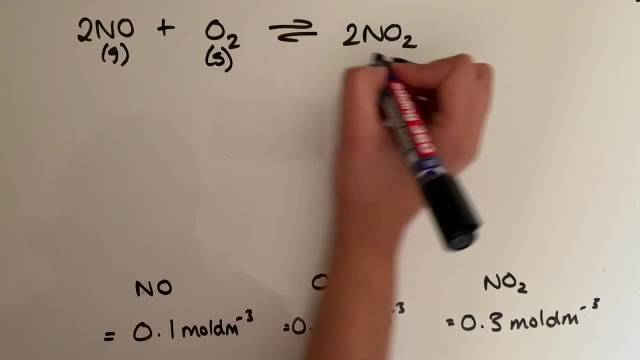 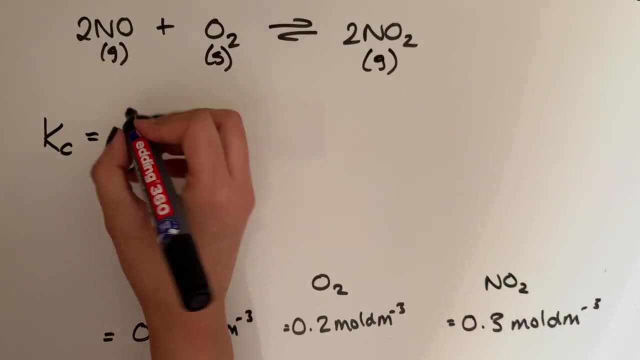 OK, these are all gases, So we can involve them all in our KC expression. It's homogenous and equilibria, So we do the products at the bottom, So it's concentration at the top, Sorry. Concentration of the products raised to their balancing number. 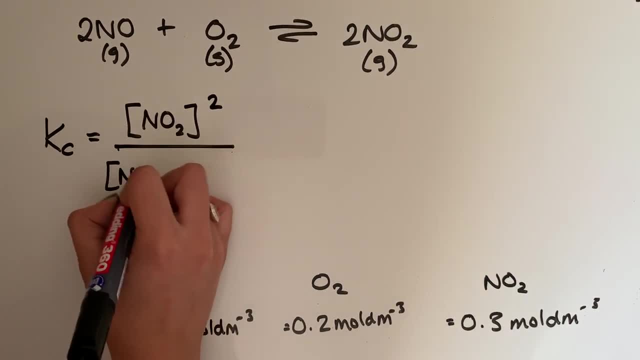 And NO raised to the power of 2 and O2 raised to the power of 1 at the bottom. OK, all we're now going to do is plug in these numbers into our KC expression. So it's the concentration of NO2 squared.